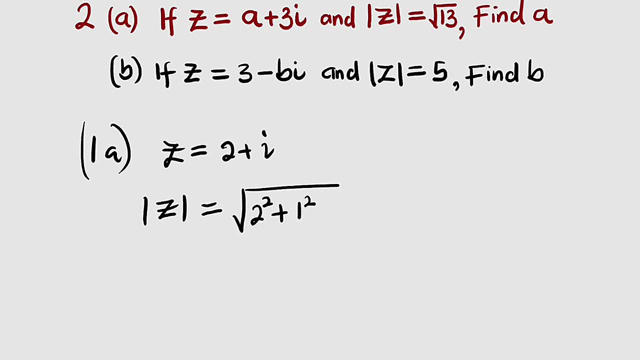 is the coefficient of I, which is 1 squared 2 squared is 4.. 1 squared is 1.. So 4 plus 1 is 5.. So this turns out to be square root of 5.. As simple as that. 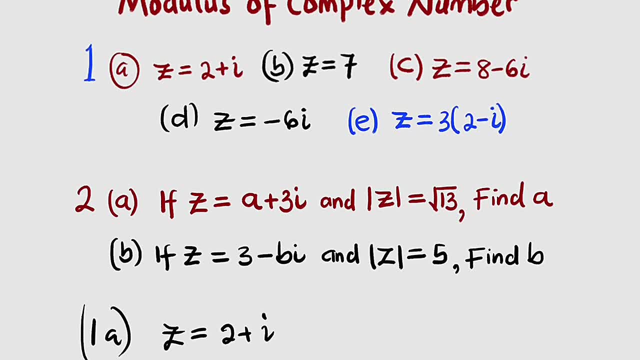 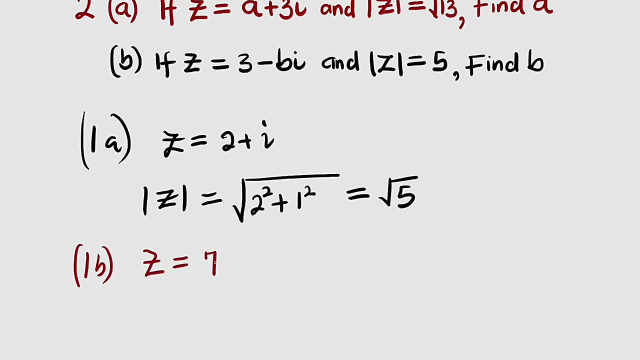 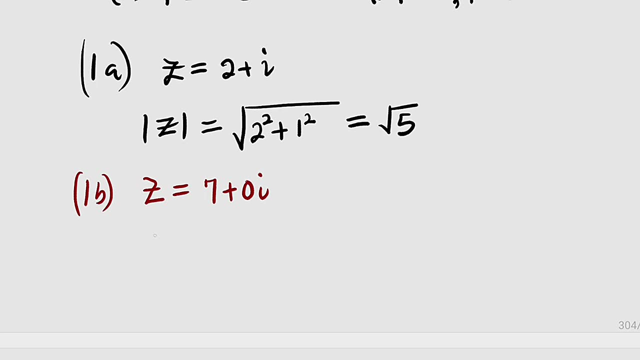 Then let us take the second one. We have Z equal to 7.. Z equal to 7, which is the same thing as 7 plus 0 I, because the imaginary part is 0.. So Z modulus, or the absolute value of Z, is equal to the square root of 7 squared plus. 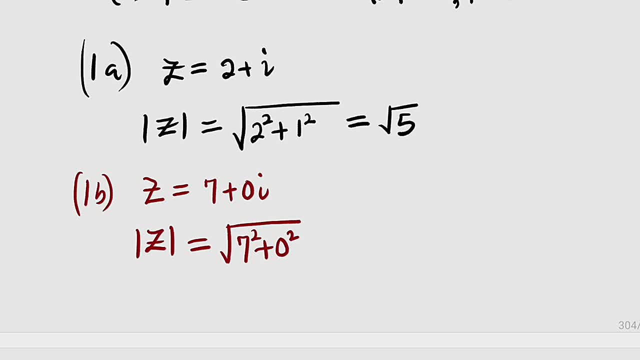 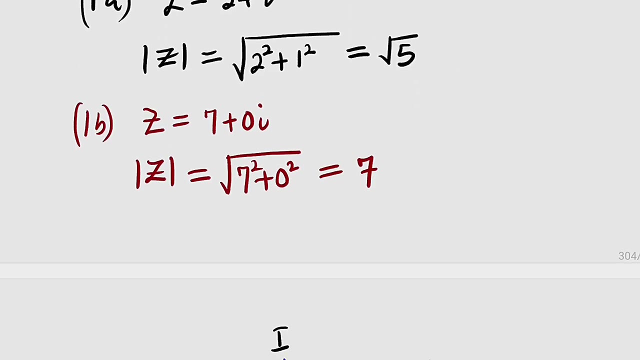 0 squared 7 squared is 49.. 0 squared is 0.. 49 plus 0 is 49.. Square root of 49 is 7.. So this is equal to 7.. Then 1C, We have Z equal to 8 minus 6I. 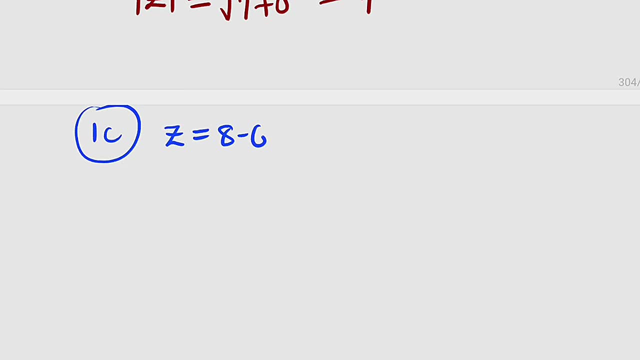 1C, Z equals to 8 minus 6I. Therefore, Z modulus is equal to the square root of 8 squared plus negative 6 squared. Let me simplify this a little bit. So 0 squared is 64.. We have 64.. Negative 6 times negative 6 is 36.. 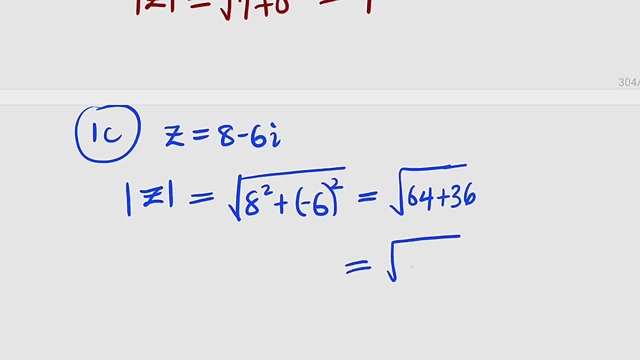 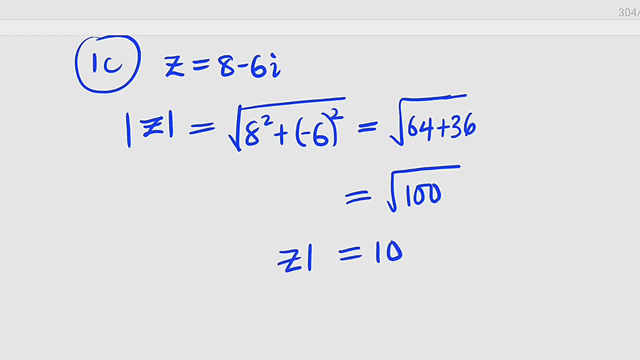 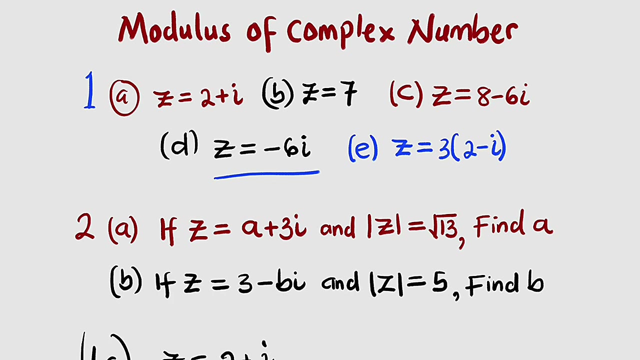 Combining these together, you have 100.. So this is 100.. And square root of 100 is equal to 10 and therefore Z modulus is equal to 10.. So I want you to try the rest of these two questions. We have Z equal to negative 6I. 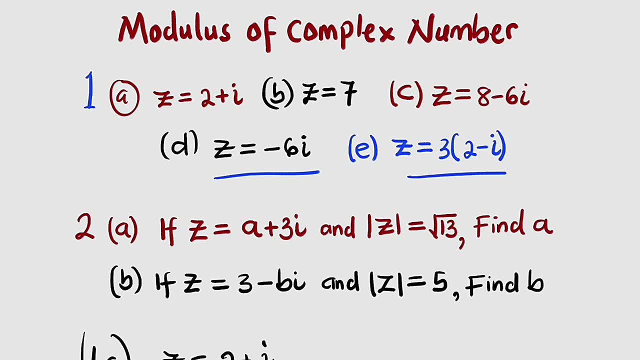 And we have Z equal to 3 × 10.. So 3÷10, which is zero, and 6I. Now let us see the rest of these two questions. One second: Yes, by 2 minus i. The only hints I'm going to give you here is that here we have 0 minus 6i, which. 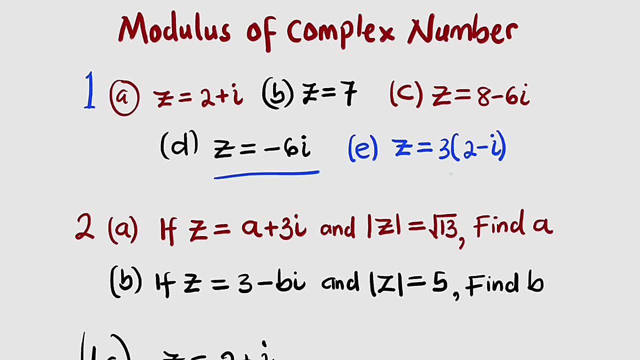 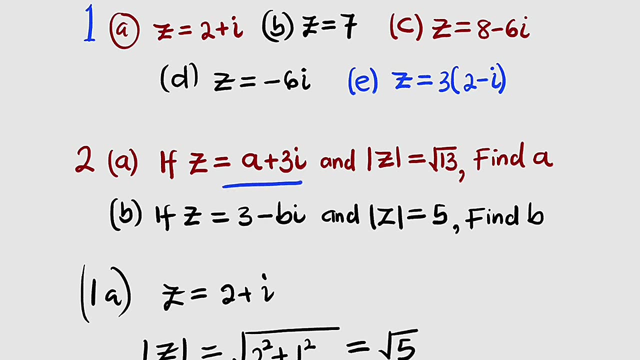 implies that the real part is 0 and the second one. you have to expand this parenthesis: 2 multiplied by 3 is 6,, 3 multiplied by i is 3i, before you take the absolute value. So we have another question here that stated that if z is equal to a plus 3i and the modulus is what square root of 13.